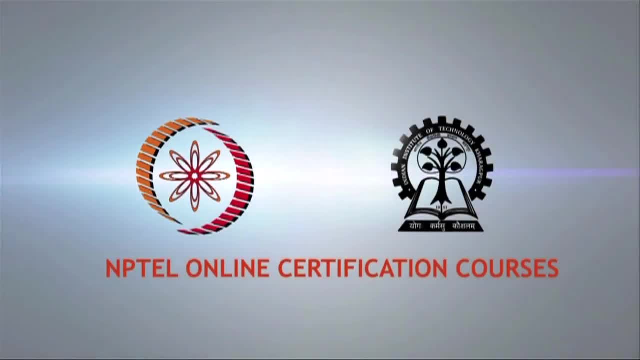 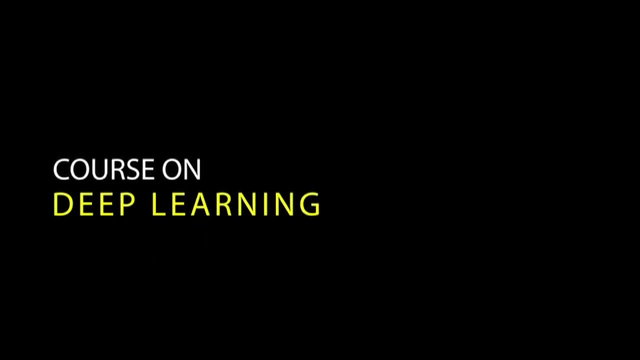 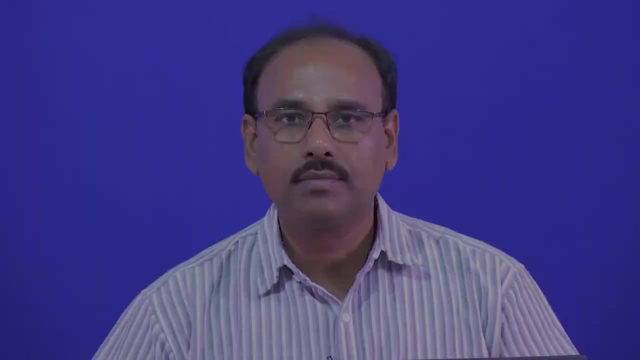 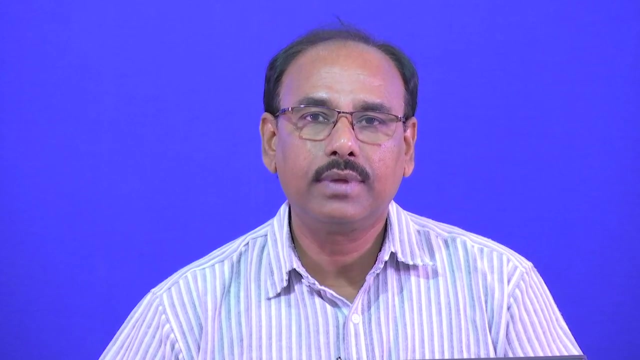 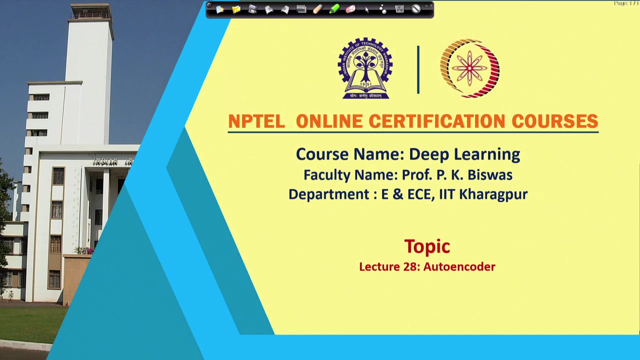 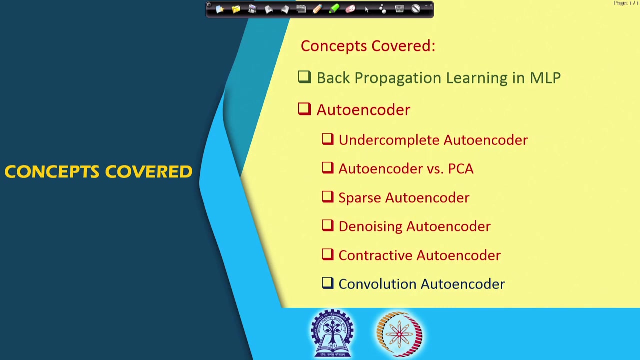 Hello, welcome to the NPTEL online certification course on deep learning. Till our previous class, we have talked about the back propagation learning and we have seen that how the back propagation learning is actually implemented or takes place in a feed forward neural network at the network level, and also how the gradient 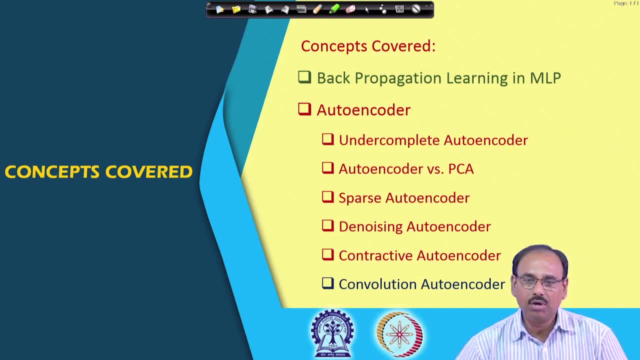 is back propagated within a particular node, or different layers or different circuits within a particular node. And, as we said in the previous class, now onwards I will assume that you know back propagation learning and whenever the learning isdiscussed I will simply refer that back propagation learning algorithm is used. I will not go into details of the 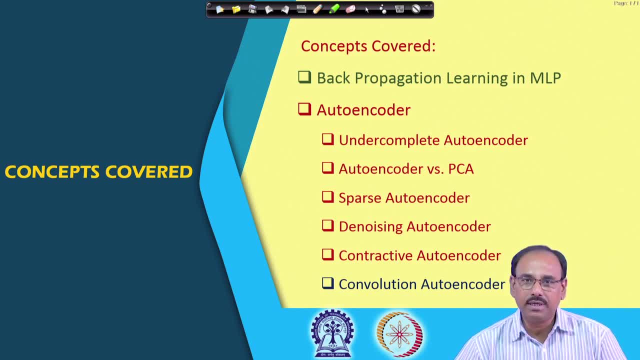 learning algorithm until and unless some details is essential. So in today's discussion we are going to start to discuss on auto encoders. So today and subsequent few lectures we will talk about under complete auto encoder, We will try to find out what is the relationship between 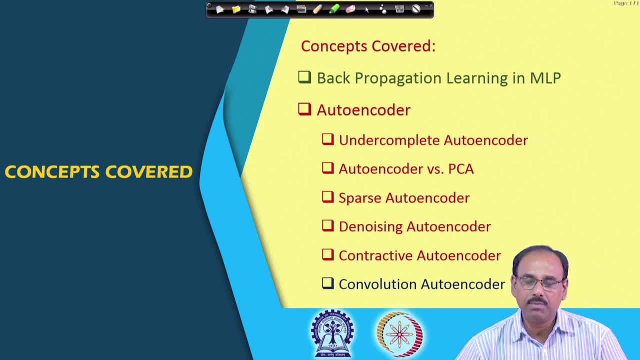 an auto encoder and a principal component analysis or PCA. Maybe I will discuss something about PCA for those of you who are not aware of this: variants of the autoencoder, namely sparse autoencoder, denoising autoencoder, contractive autoencoder and so on. And then we will also talk about convolution autoencoder, but not. 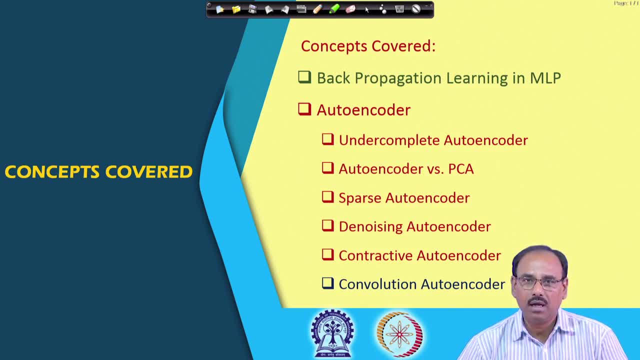 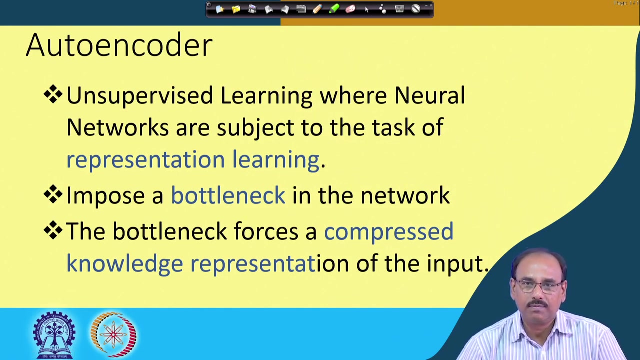 as a continuation of thisseries on autoencoders, but we will come back to convolution autoencoder after we discuss about convolution and convolution neural network. So today, what we are going to talk about the autoencoder and under complete autoencoder. Now what is this autoencoder? As the name suggests that autoencoder is nothing but. 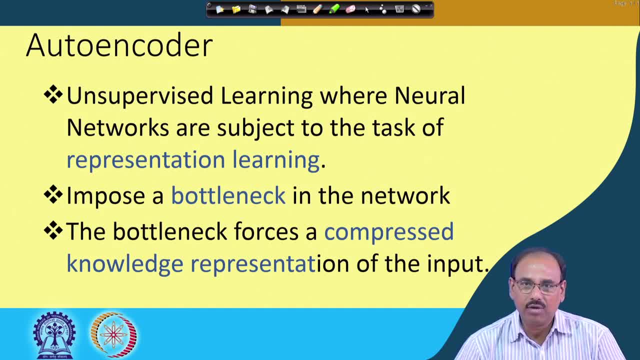 an algorithm that codes itself or that encodes itself. So you can say that autoencoder is a self-coding algorithm. So you can say that autoencoder is a self-coding algorithm. So you can say that autoencoder is an unsupervised learning algorithm where the neural networks 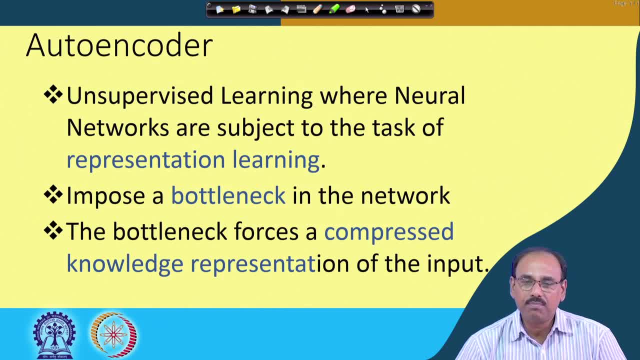 are subject to the task of representation learning. And what is this representation? The representation is nothing but how you code or how you encode the input data that is fed to the network. And learning this representation, learning this code, is what is known as neural. 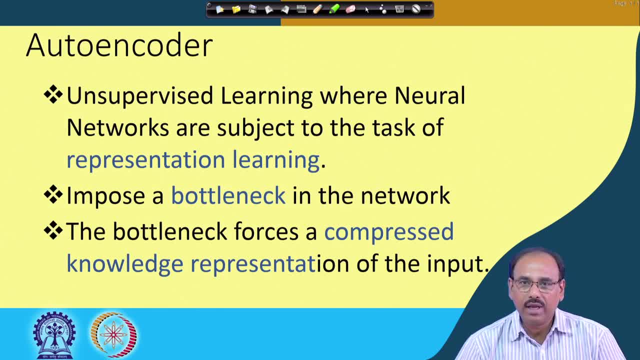 representation learning, And we say autoencoders are unsupervised learning, because when you train an autoencoder for coding an input or forencoding an input, we do not use datas which are level datas, unlike in case of classification problems that we have discussed earlier. So 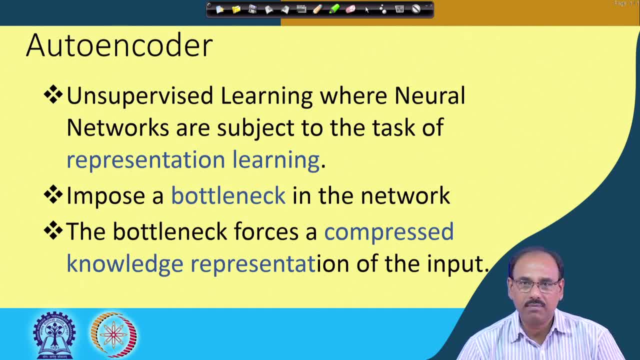 if you remember what we discussed in case of classification, that for training the network or for training of your classification. So you can say that autoencoder is a self-coding classification algorithm, machine learning algorithm. we need a lot of training data. 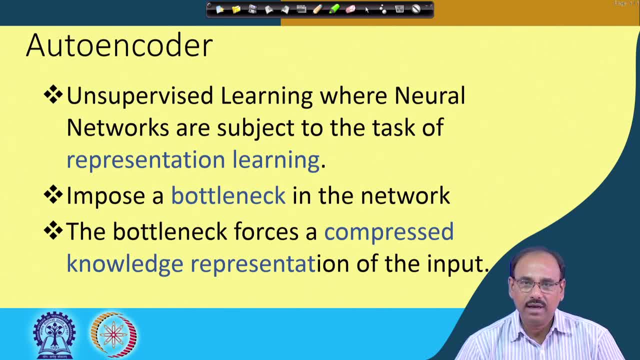 And what that state of training data tells you is that it tells you that what is the class belongingness of a particular training data And it is only from that information of class belongingness I can compute the error, Because if my machine says that a training 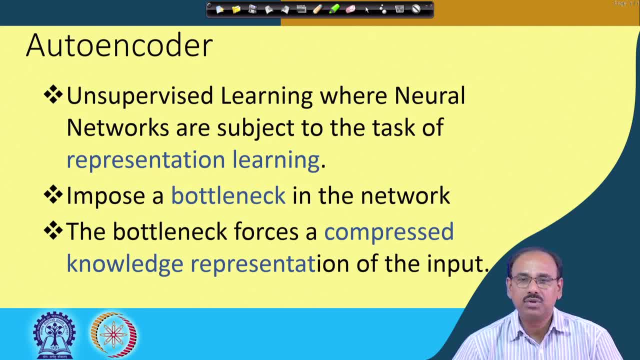 data, or if my machine infers that a training data belongs to some category, say 5,, what is the error? Whereas the ground truth says that that particular training data belongs to category 1. So there is a mismatch. my machine says it is category 5, whereas the 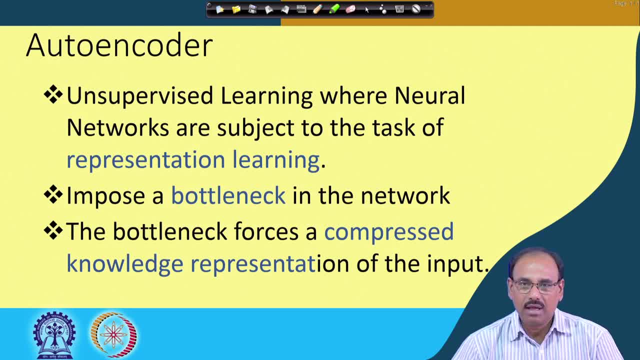 ground truth is category 1.. So there is an error and your learning algorithm, as we said, using back propagation, tries to minimize this error. That means, as the machine has interpreted to be 5,. what modifications or what updations in the weight vectors we 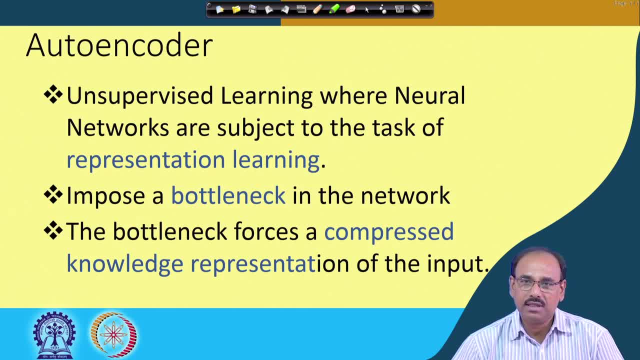 have to do So that the machine really interprets this data to belong to category 1.. So those are the supervised learning algorithms, because the data that is used for training or learning are the leveled data, But in case of autoencoder, the data that we use are not leveled data. 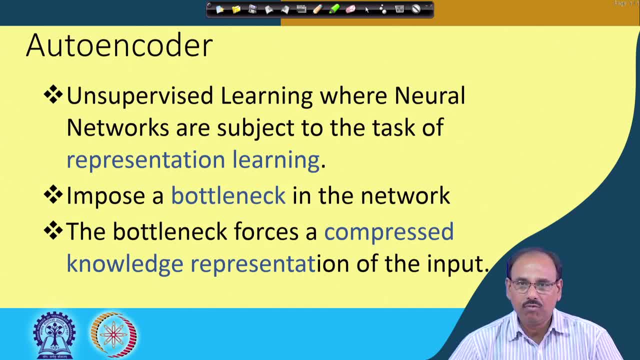 However, we still have back propagation algorithm because we want that. whichever way the machine represents or the autoencoder represents the input data, from that representation it is possible, it should be possible, that we should be able to reconstruct the input data. That means I have to find out that after encoding, whether the encoded data can be reconstructed. 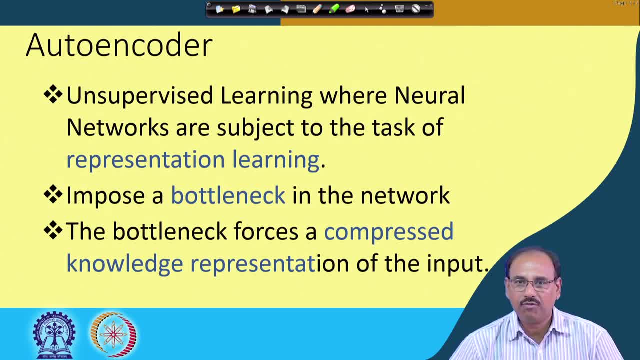 So if for encoding I call it a forwardencoding algorithm. So some mapping function f that gives me the encoded data, Then another mapping function g should be able to convert or transform that encoded. 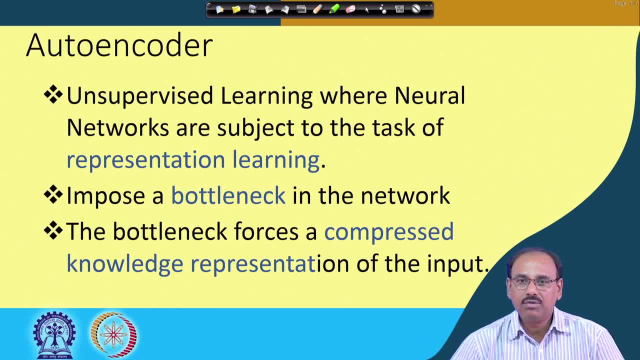 data to my original input And for learning. what you do is you compare the original input and this reconstructed input and try to minimize the error between these two. So this autoencoder, as we said that it is an unsupervised learning and the task of the 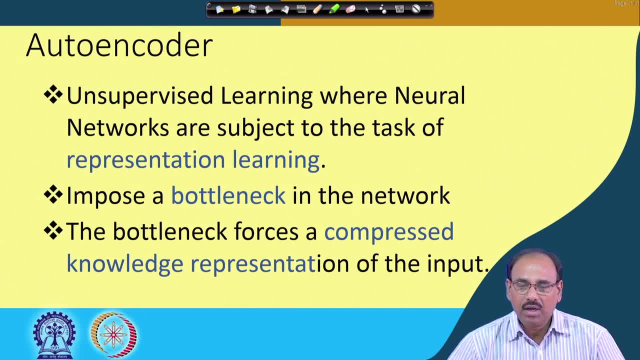 neural network, in this case, is to go for representation learning, or try to encode, or learn how to encode or how to code the input data. And in order to do this, what you do is you introduce a bottleneck in the network Because, as we said, that our learning algorithm will. 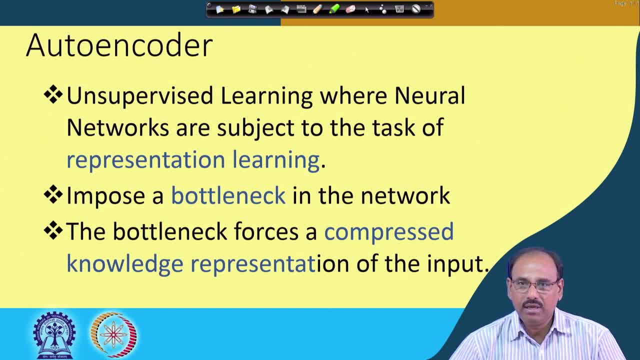 be that I have an input, I have some coding in between, then I have a reconstructed output And I want that the reconstructed output should be similar to the input, or they should be identically possible. So there is a possibility that the network 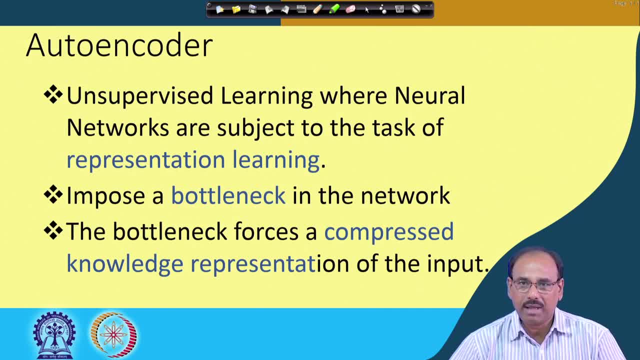 may eventually learn an identity mapping. ok, So if the network learns an identity mapping, it does not learn, it does not really learn the representation. So, in order to enforce or in order to force that the network learns the representation, or network learns what, 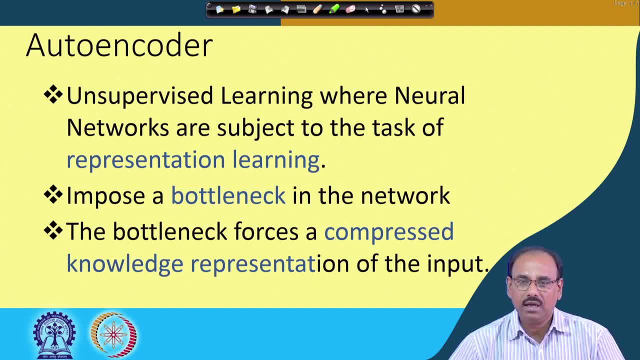 is the inner structure of the data. it is necessary that in the network you impose a bottlenecklayer. So we will come to a bit later details of how this is done. And this bottleneck actually forces a compressed knowledge. representation of the input. That means, if my input vector 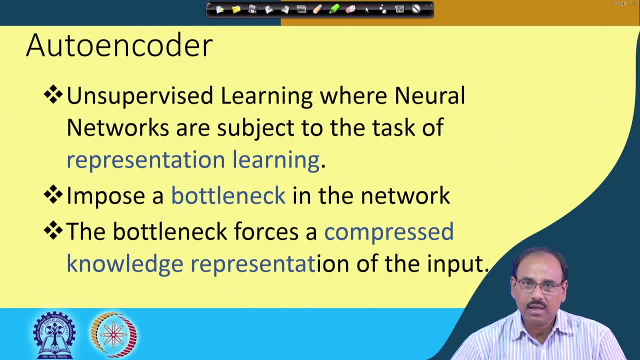 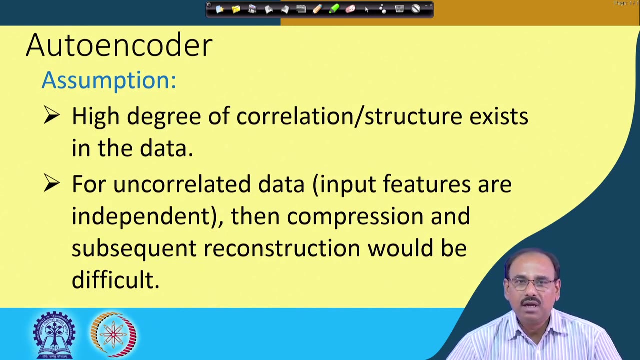 input data is of dimension, say d. in this compressed knowledge representation it will be mapped to a vector of dimension, say m, where m is much, much less than d. So how it is done, we will come to this a bit later. So for this we have certain assumptions. The assumption is there is a high degree of 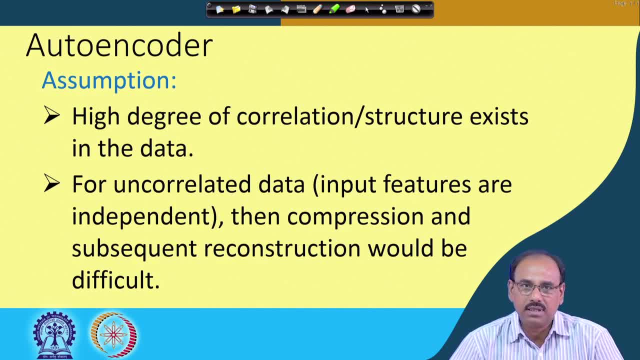 correlation or structure that exists in the data. If the components of the input data are not correlated- that means if the features are independent of one another- then this compressed domain representation and subsequent reconstruction of the original input will be difficult. In fact, it may not be possible at all. 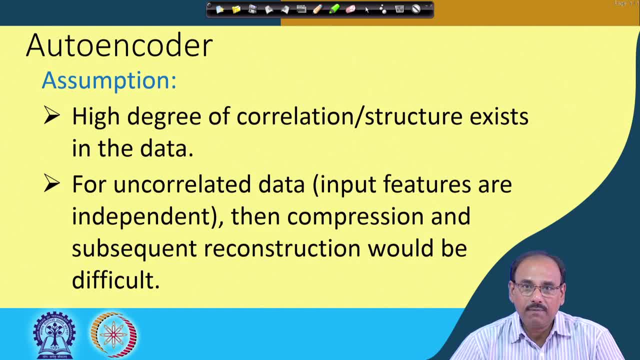 So when the neural network goes for representation learning or tries for representation of the input data in compressed domain, what it tries to do is It removes the correlation of the redundancy present in the data, And what is what it preserves is only the uncorrelated. 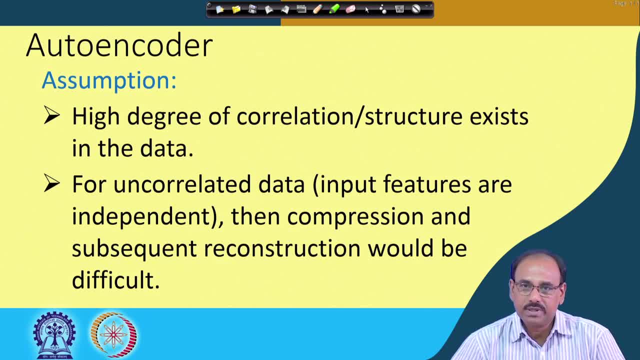 part and from this uncorrelated part, then it should be subsequently possible to reconstruct the original input data. So that is what an autoencoder is and, as we said that the name autoencoder indicates that it encodes the data or it codes the data on its own. 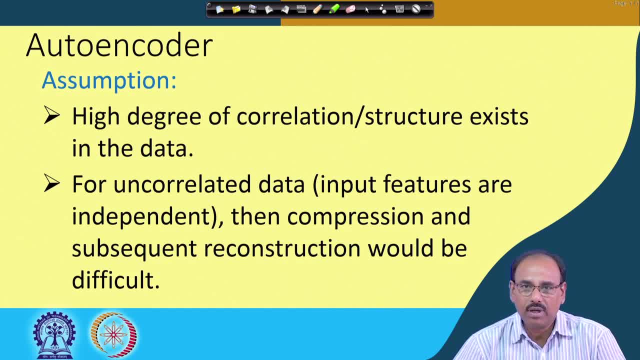 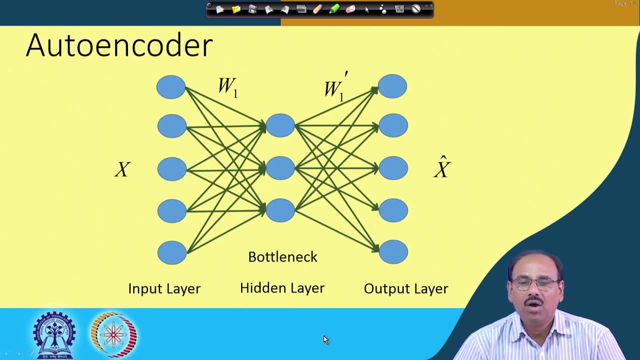 And this is an unsupervised learning, because for training an autoencoder we do not use any label data. What we want is: whatever is fed to the input, the autoencoder outputs the same thing. So for this I need two different functions. one is the encoding part, one is: 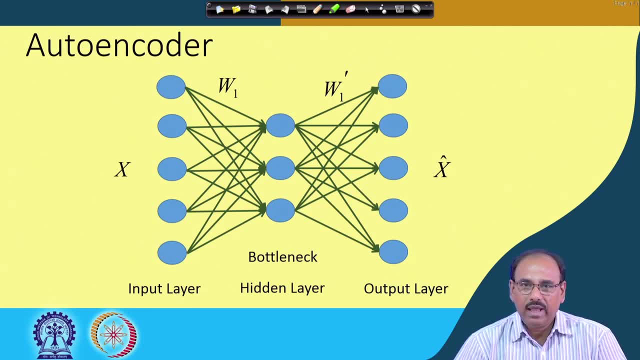 the decoding part. So the encoding part will encode the input data to ancompressed domain representation, knowledge representation, and the decoder part will decode the data from that compressed representation, from theencoded output, to your original outputorginal output. So if my input was x, it will reconstruct x hat. I want that x and x hat should be similar. 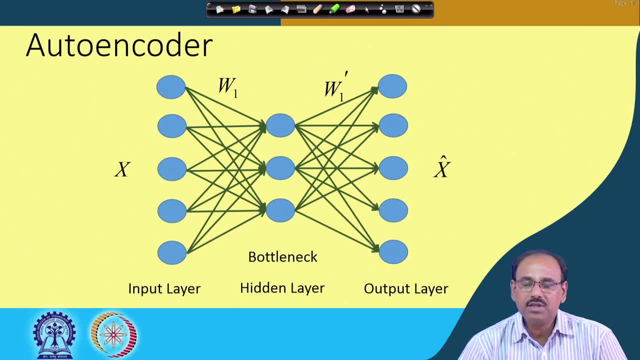 or the error between x and x, hat should be minimum and that is what is given by the decoder part. So I should have an encoder half, I should also have a decoder half and this is the structure, thebase structure of an autoencoder. So you find that in this autoencoder I have 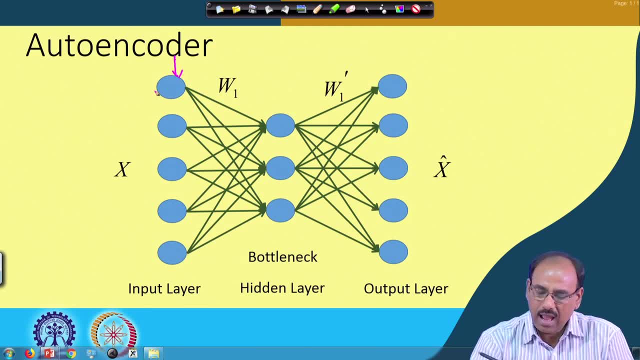 an input layer. this is the input layer and I have a hidden layer and I have an output layer. So this hidden layer is actually the bottleneck layer. So in the bottleneck layer, what you are doing is you are compressing the data. you are going for compressed domain representation. So you find that the number of nodes in the 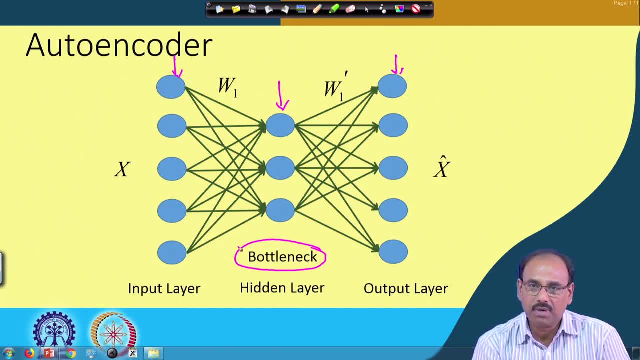 hidden layer, or the number of nodes in the bottleneck layer is much less than the number of nodes in the input layer. And also you find that the number of nodes in the input layer is same as the number of nodes in the output layer because, finally, 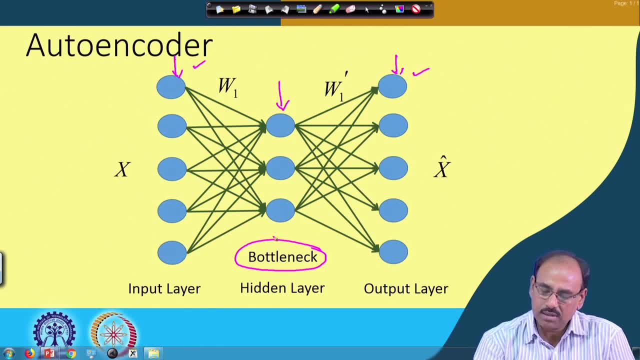 at the output. I want that, whatever was the compressed domain representation in the hidden layer from this compressed domain representation, it should be possible to reconstruct my original input. So original input was x. I should be able to reconstruct this x, which is x hat. So obviously the dimensionality of x and the 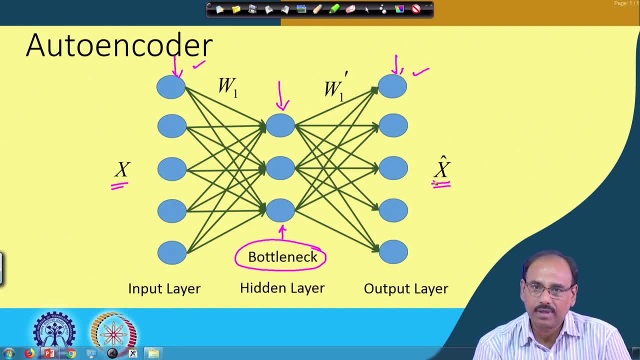 dimensionality of x hat should be same. So what does it mean? Say, for example, I use this network for compressed domain representation of an input image and suppose image is of size m by n. So there are m into n number of pixel. 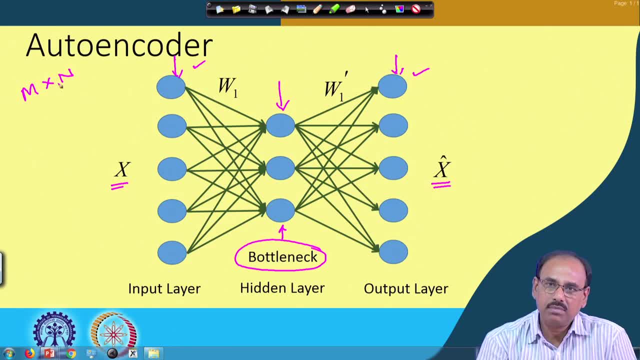 So, as we said before, that by column concatenation, this m by n matrix can be represented by an one-dimensional vector use, having m into n number of elements. that we have to do by column concat concatenation. So if each of the n, each pixel, is fade to one of the nodes, 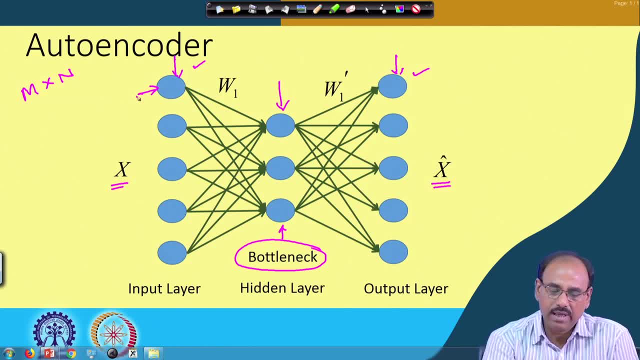 on the input layer. So the number of nodes in the input layer has to be m into n, because every node input in the input layer gets 1 pixel. In addition, we have to have one more node to represent the bias. so the number of nodes in the input layer has to be m into n plus 1.. Whereas on the 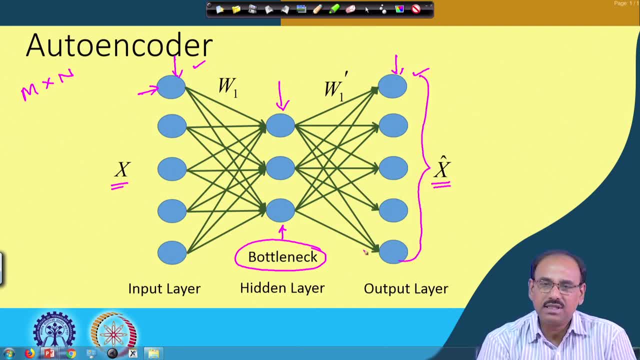 reconstruction side. I do not need any bias, I just want my x back. so that is what I need: an x hat. So the number of nodes in the output layer has to be m into n as against m into n plus 1 on the input side. Now suppose I want that, this entire image. 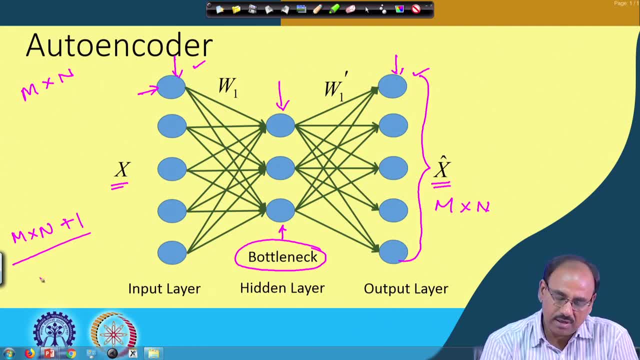 should be represented by a d dimensional vector or a vector having d number of components, where d is much less than m into n. So in that case the number of nodes in the hidden layer has to be equal to d, which is my bottleneck layer, but the reconstruction purpose I need. 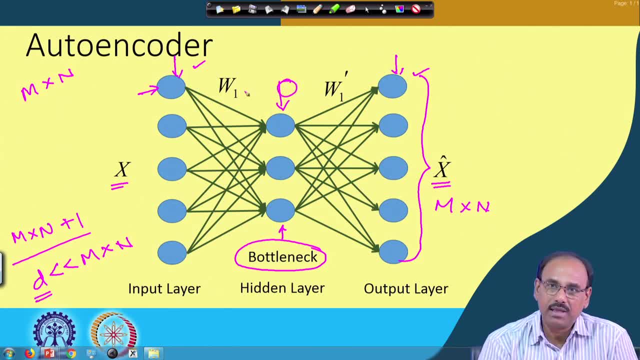 1 more additional node to take care of the bias. So the number of nodes in the hidden layer for the decoding side or for the reconstruction side, will be m into n plus 1. So the number. So this is the base architecture of an autoencoder. Now you find that. so I have an input layer. 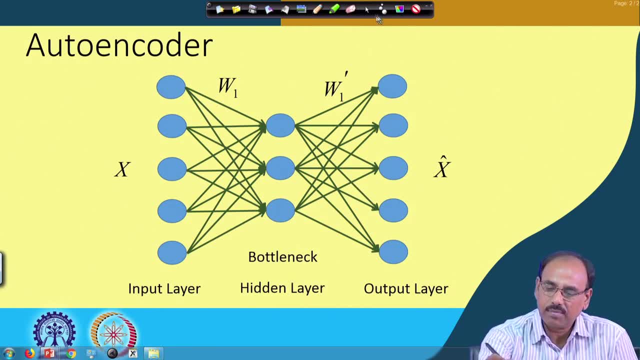 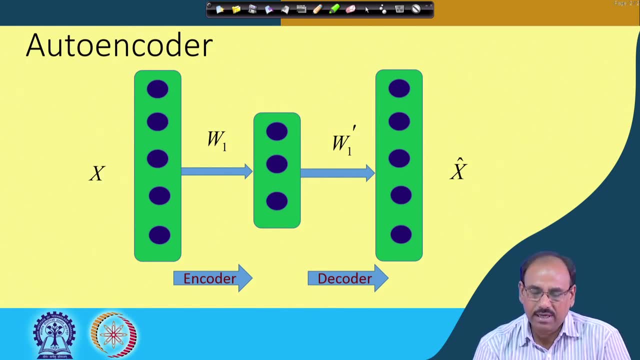 I have an output layer, I have an hidden layer or a bottleneck layer. Now this same architecture now onwards. for simplicity, I will represent like this: that input layer will be an array of nodes, hidden layer will be another array of nodes, where array of array size in the 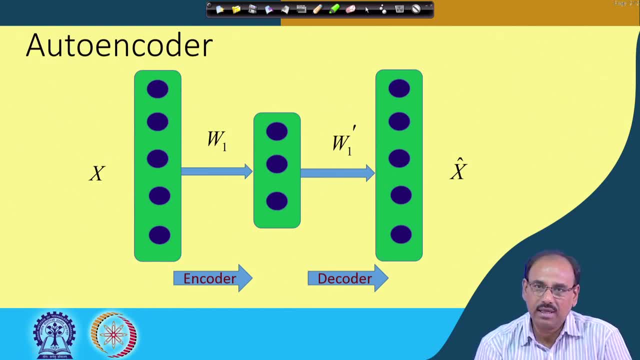 hidden layer will usually be less than the array size in the input layer. Similarly, on the output side also, I will have an array of nodes and I will have a set of weights, say W 1 and W 1 dash. So this W 1 connects the input layer to the hidden. 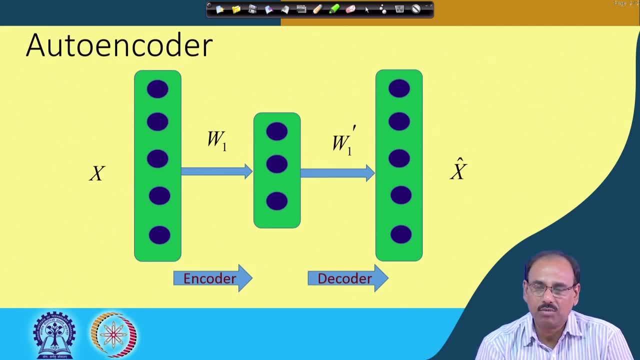 layer and W 1 dash connects from the hidden layer to the output layer. A right: it is also possible that instead of having just one hidden layer, I can have multiple hidden layers. Now, before that, this side, when you are going from input to the 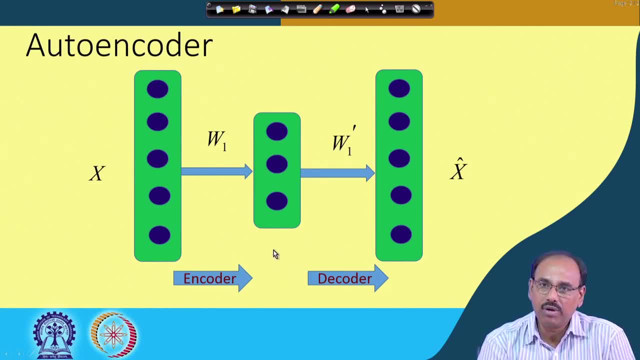 hidden layer. the hidden layer actually gives you the encoded information in a lower dimension in general. Later on, when we talk about sparsity or sparse autoencoder, we will see that it is not necessary that I will have to go for dimension. I can have a similarity reduction. I can have a dimension explosion as well, or maybe of. 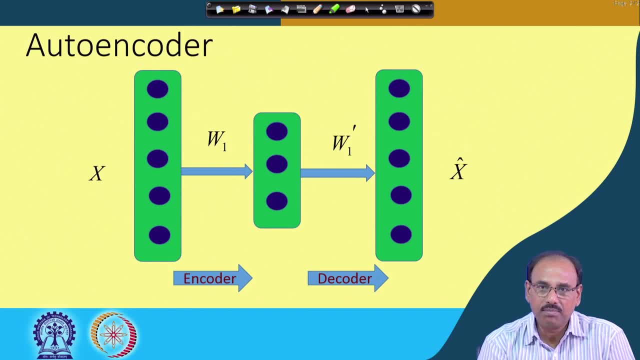 the same dimension, but there your compressed representation is done by some other mechanism. However, for the timing, let us assume that we are going for compressed domain representation, knowledge representation. So from input to the reduced dimensional representation, that is a part which is the encoding part. So this is the encoder side. 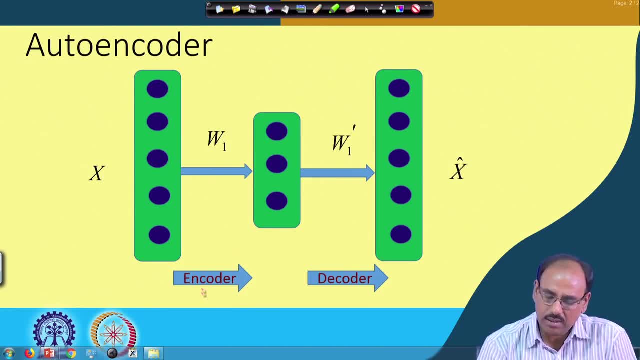 So this is what is your encoder. and similarly from compressed domain representation to the reconstruction of the original signal. this is what is the decoder part. So I have an encoder, I also have a decoder. It is also possible that I may not have only. 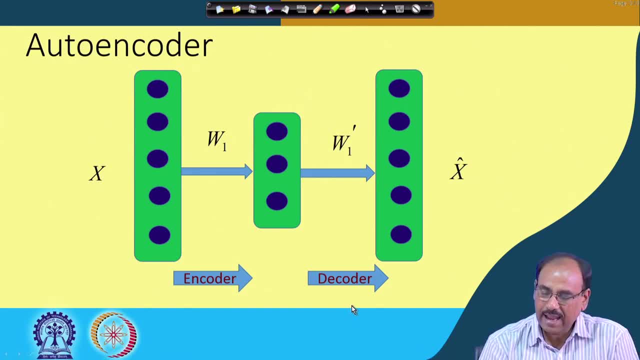 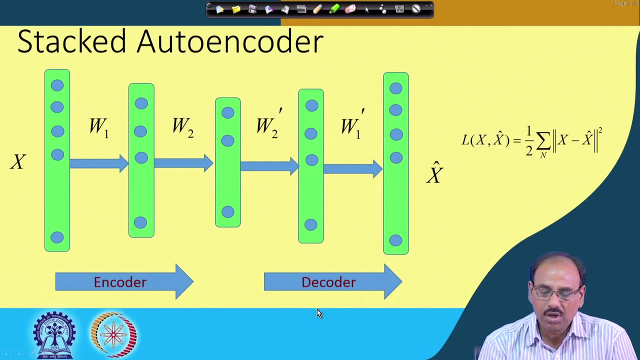 one hidden layer or only one bottleneck layer. I can have multiple number of hidden layers So I can have aeverast of it. you know, even in sort of anуль plane or mistakes have a situation something like this. So on the encoder side I have a number of hidden. 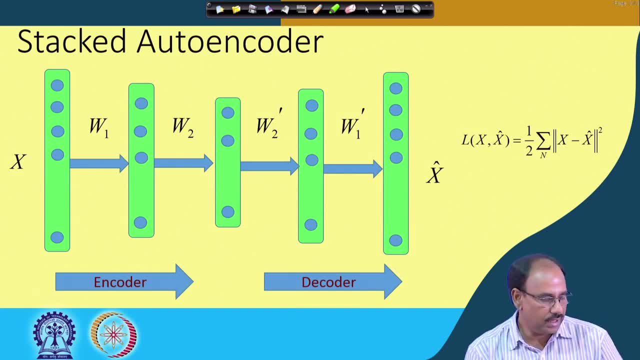 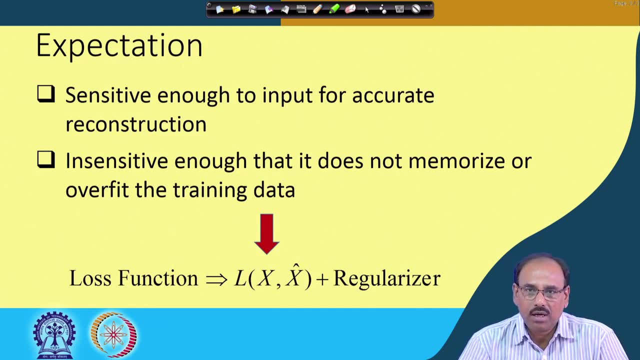 layers. on the decoder side also, I will have a number of hidden layers. I will come back to this one a bit later. Now, in this case, as we said that when I have an autoencoder, what I have is I have input data and output of the autoencoder is also a data, and I want 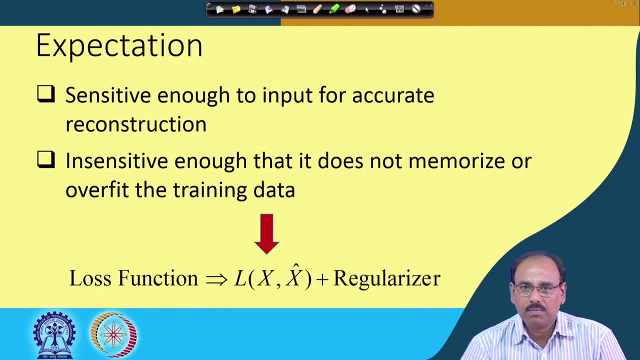 that the output should be a faithful reconstruction of the input, And while doing so, the information passes through the bottleneck layer, where, in the bottleneck layer, I have a compressed domain representation or coded version of the input data. Now I my expectation from such an autoencoder is twofold. Firstly, I want that the auto encoder should be the same as the input data. So the input data should be the same as the output data. So the input data should be the same as the input data. So the input data should be the same as the input data and the autoencoder should be sensitive enough. 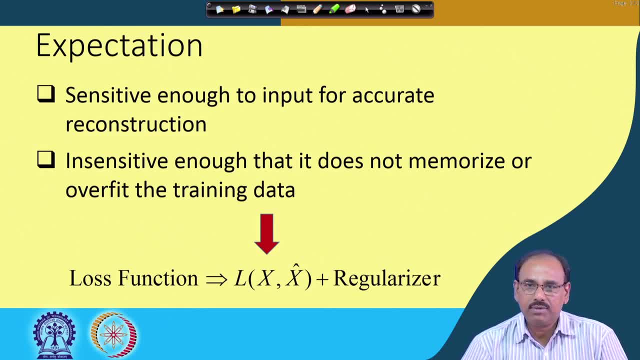 to the input for accurate reconstruction. Because what we said is my reconstructedvector x hat should be as close as possible to input x. So that means my autoencoder should be accurately, should be able to accurately reconstruct my input signal. So that is what is it is. 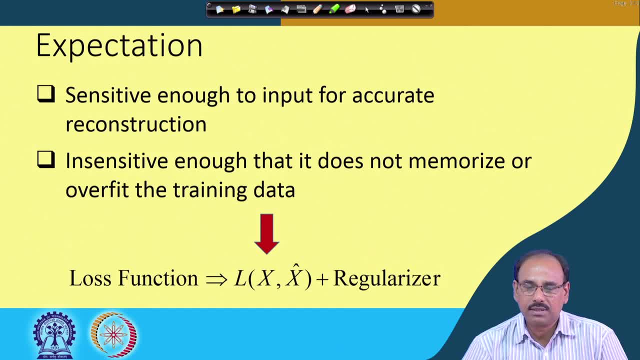 sensitive enough to input for accurate reconstruction. Now, if accurate reconstruction is my aim, not the representation, then an identity function is sufficient. So it might be possible that autoencoder simply learns the identity function. So if it simply learns the identity mapping, it will always reconstruct your output faithfully. 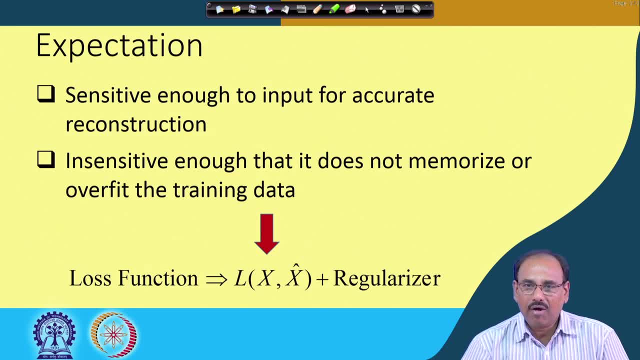 as the input, but that is not our aim. Our aim is actually what is happening at the bottleneck layer. that is, how the input data is represented in in the compressed domain. that is what is my interest, And this encoded data will be useful for some later applications, because 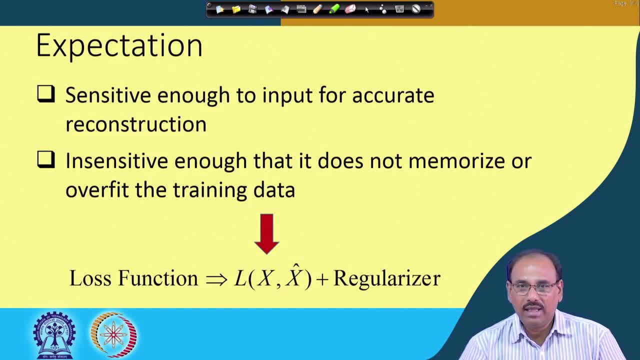 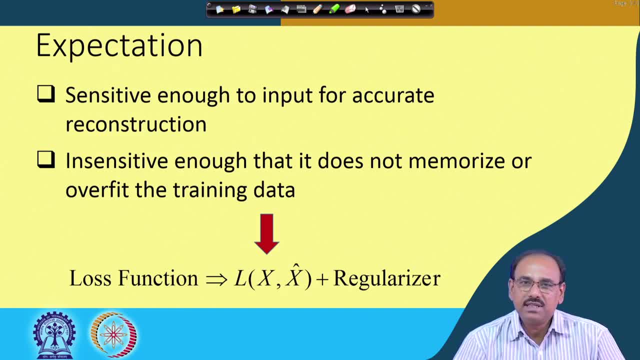 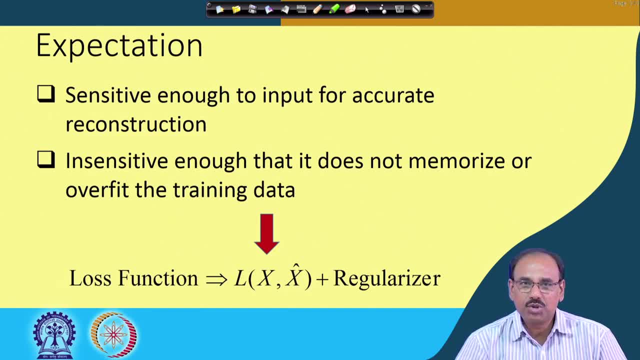 that it should be sensitive and, at the same time, it should not be sensitive enough. So how do you impose or how do you try to satisfy both these requirements, both these conflicting requirements, simultaneously? So that is actually done by designing your loss function, which takes care of both of them And this loss function, as we said that. 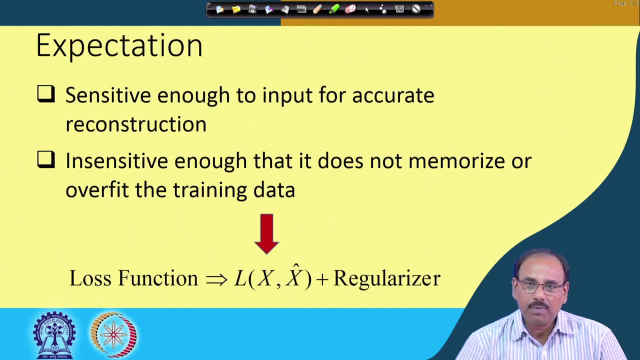 the loss function will be used for back propagation learning algorithm when you train the autoencoder. So the loss function in this case will be given bythis that this loss function will. loss function will have two components. one is L X x hat, which is the error between the. 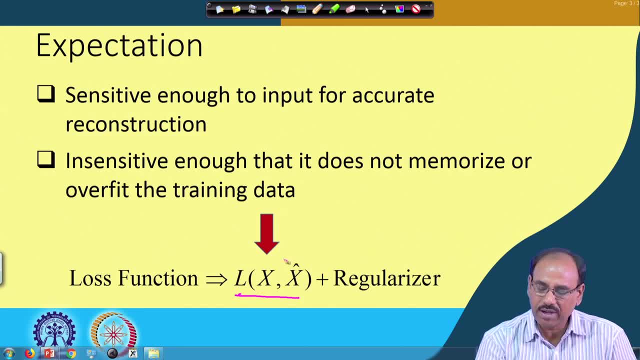 input X and the reconstructed X hat. So if I want to minimize this, so minimization of this. the error takes care of this: that the autoencoder is sensitive for faithful reconstruction of the input, Whereas the second requirement, which conflicts the previous requirement, is: 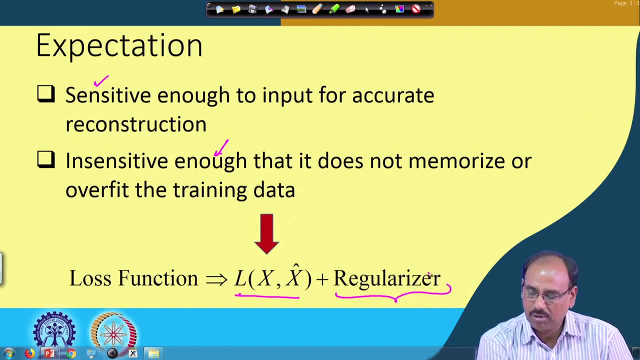 through a regularizer. regularizer term. So in the loss function you have an error function between X and X hat and you also have a regularizer term. So the regularizer term will try to make it insensitive to the input and it will force the autoencoder to learn the low dimensional. 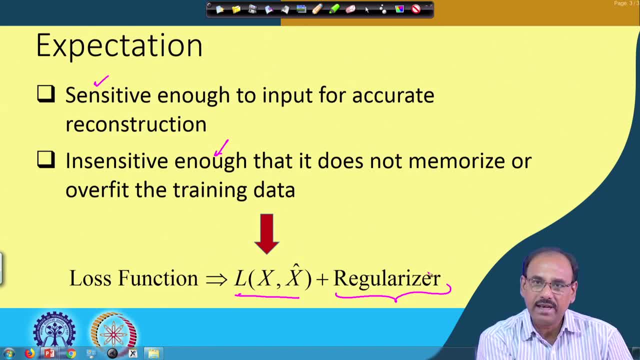 representation. So here it learns the salient features of the input, So that using the salient features, the decoder will be able to reconstruct the data. So it does not simply learn the identity function. So both theserequirements- conflicting requirements- are made, are satisfied by defining: 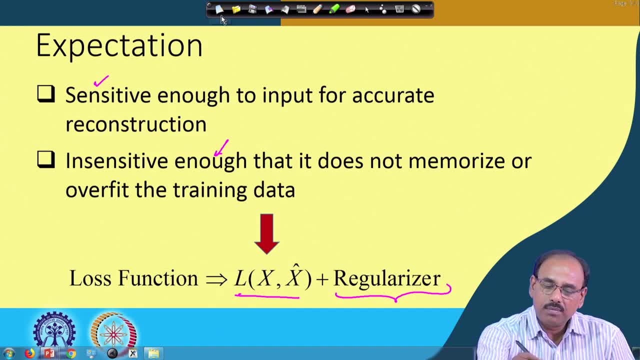 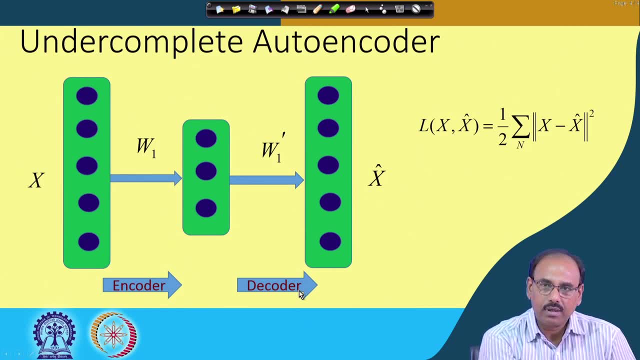 a loss function of this form. So this is what I said: thatthe way of variant of the autoencoder, which is known as under complete autoencoder, takes care of the regularization, is by introducingor by introducing restriction on the number of nodes in the hidden layer or the bottleneck bottleneck layer, So as 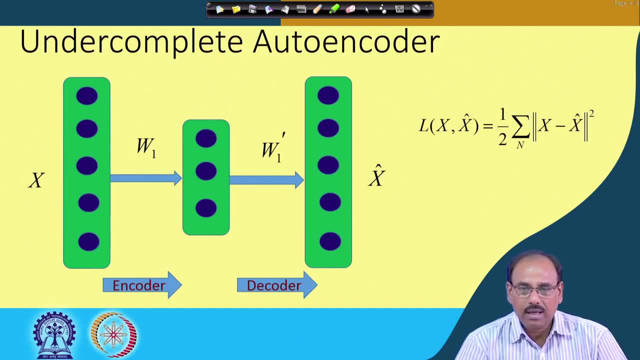 we said. usually, number of nodes in the bottleneck layer or the hidden layer is much less than 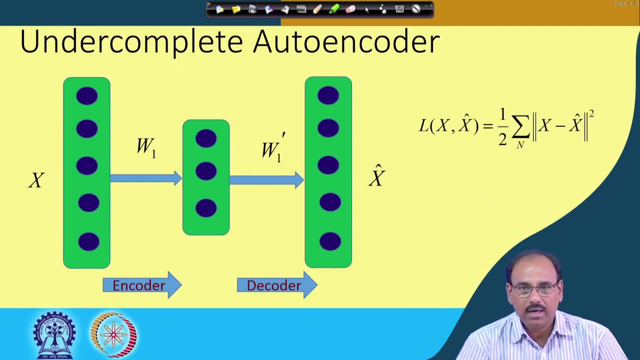 the number of nodes in the input layer or, similarly, the number of nodes in the output layer. So in such casesthe network is made insensitive to the input by restricted number of nodes in the hidden layer, And when I have an architecture of this form, this is what 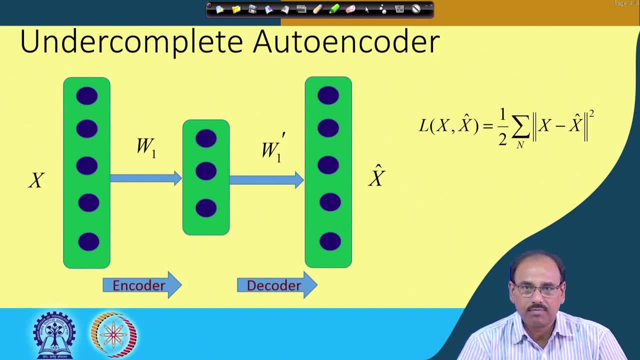 is known as an under complete autoencoder architecture, And for training such an autoencoder you simply minimize the loss function which is given by L x, x hat, which is half of x minus x hat. take the L 2 norm of that and sum of this over all the training vectors. ok. 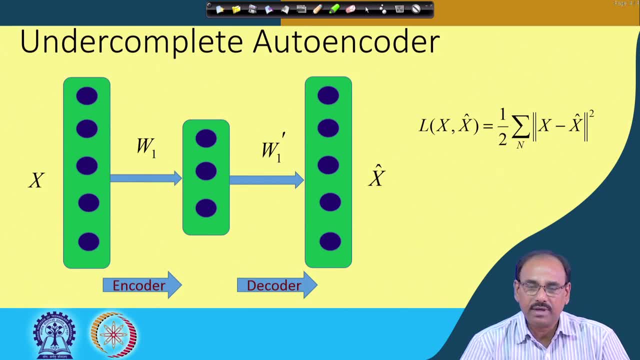 A? nd. you find that here, as we said that this is an unsupervised learning, because I do not need to have a knowledge of the class belongingness of the input vector x. What I simply only need is that the x and x hat should be similar. 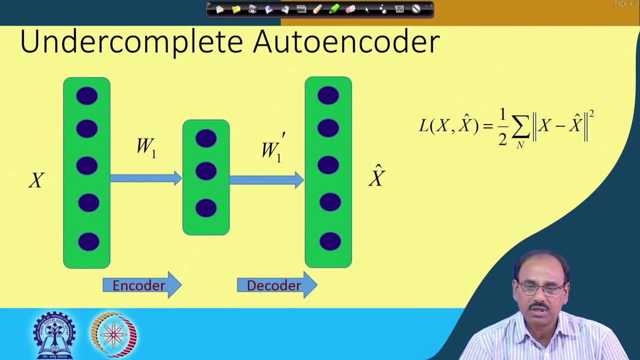 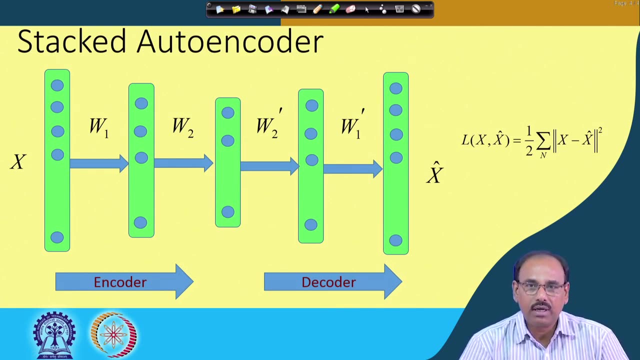 that is x. hat should be a faithful reconstruction of my input x. So this is what is my under complete autoencoder. Now, as we said before that it is not necessary thatthe autoencoder have to have only one hidden layer orthe bottleneck layer, I can. 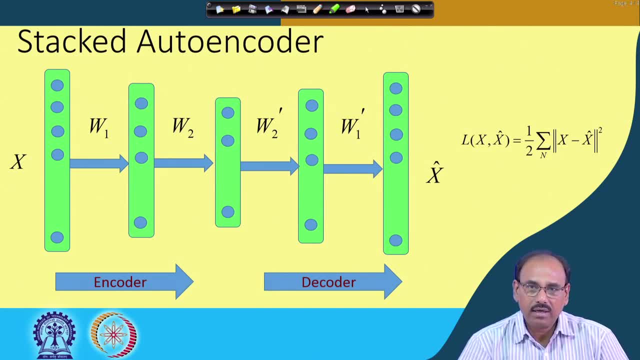 have an stacked autoencoder where a number of hidden layers are stacked one after another. So this diagram shows that I have a stacked autoencoder where obviously x isfailed to the input layer. I have the firsthidden layer in the autoencoder on the encoding side, The 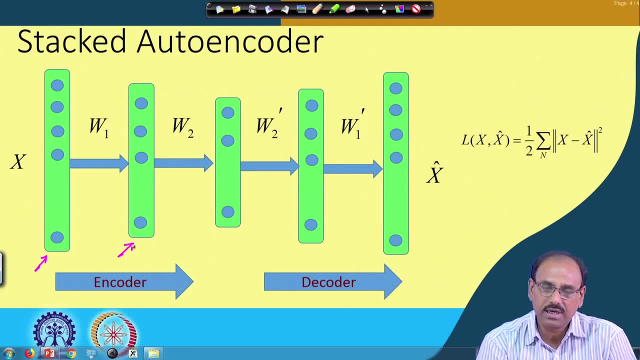 connection weights between the input layer and the first hidden layer. autoencoder layer is given by the weight vectors or weight matrix w 1.. Then I have the second hidden layer and in this case the second hidden layer happens to be the bottleneck layer. 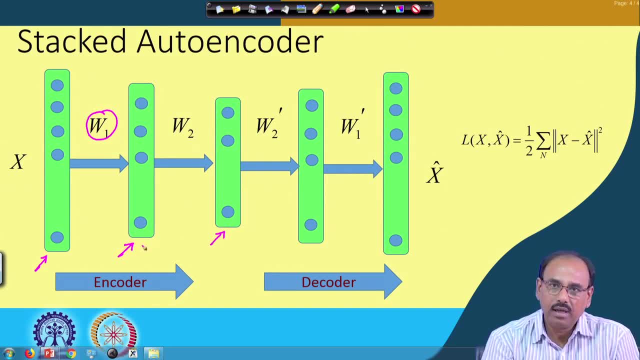 And the connection weights between the first auto encoding layer to the second hidden layer. the second auto encoding layer is the set of connection weights, W. So this completes my encoding part. Then on the decoder side, from the encoded data, it goes to the first. 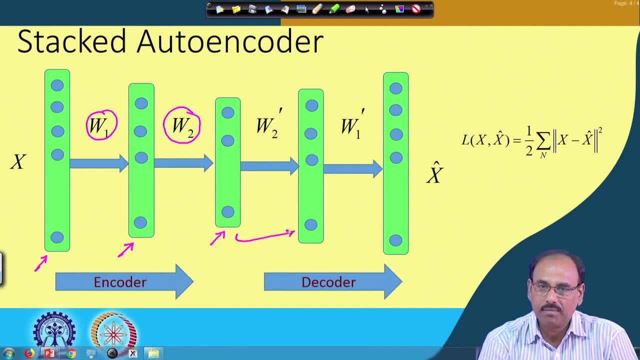 hidden layer on the decoding side and the connection weights from this to this is given by W 2 dash, And similarly, from this hidden layer to the output layer, the connection weight is given by W 1 dash, And what I simply want is that 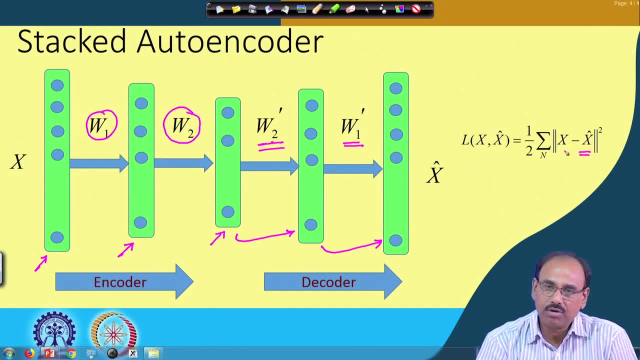 the x hat should be a faithful reconstruction of x. that is the input error And for that the loss function that you have to minimize is the L 2 norm between L 2 and L 2.. So this will be equal to son or x hat And this has to be summed over all the training data. 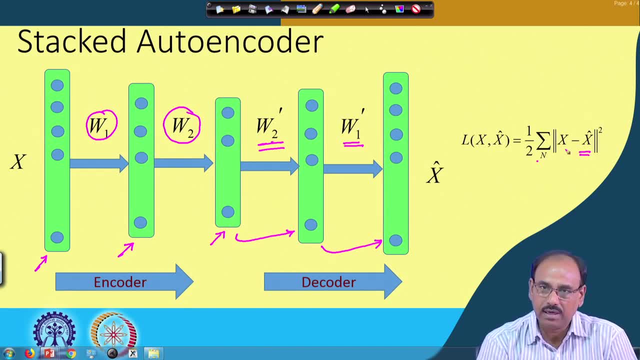 and you minimized this L 2 norm using back propagation learning algorithm And while this is minimized, you find that this weights W 1, W 2. similarly W 2 dash and W 2, W 1 dash. they will be modified. they will be updated until and unless the L 2 norm or the error 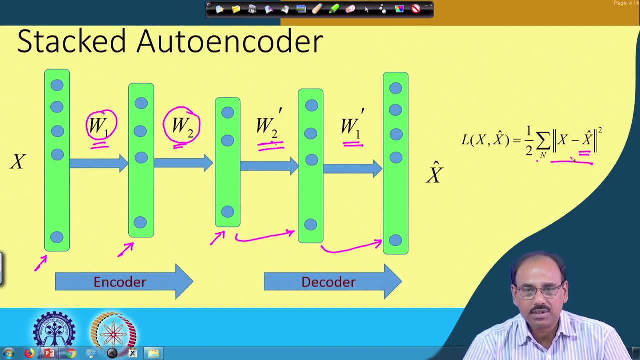 between X and X. hat is 0 to x, So that is going into the inilikting And 0 or it is within an acceptable limit. At that point we say that my auto encoder is properly trained. Now what you do after the auto encoder is: 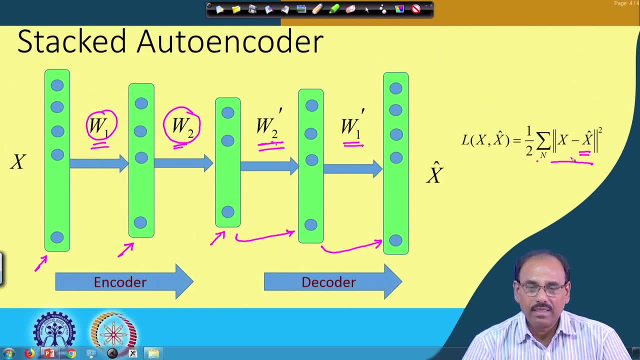 properly trained. I said earlier that reconstruction is not my aim. I want to reconstruction. I want to reconstruct the input data from the encoded data, just to ensure that my encoding is proper. That is whatever my is my encoded data from the encoded data? I should be able.